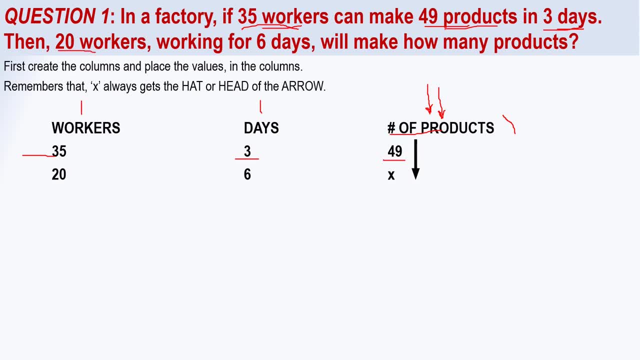 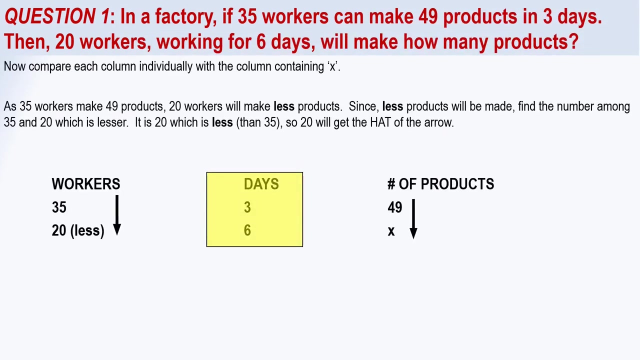 number of products. Similarly, we are given that 20 workers, So we write it here. then in six days, So they do it here. We do not know the number of products that they make, So we denote it by X. So in the second step we shall draw arrows for the other columns. So we have other columns. 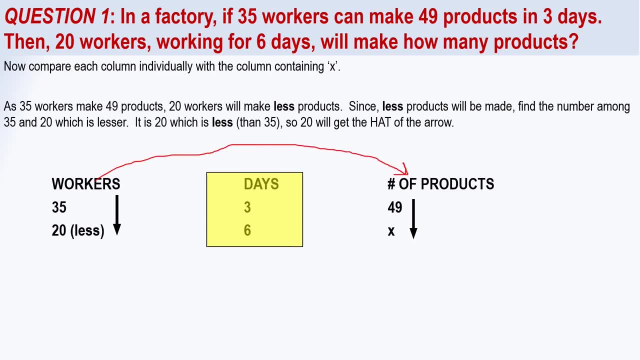 as workers columns, And we shall compare it with the column containing unknowns. And while we do that we will not worry about the other column which is days column. So we have kind of shown it as hidden. So we will compare the columns individually. So we have here in this column as workers 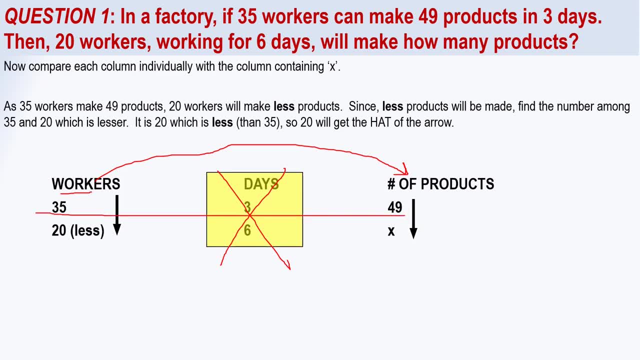 we see that 35 workers produce 49 products, Then 20 product 20 workers will produce how many products it is? it will be less products because 35 are only producing 49 products, So 20, which is less number of workers. 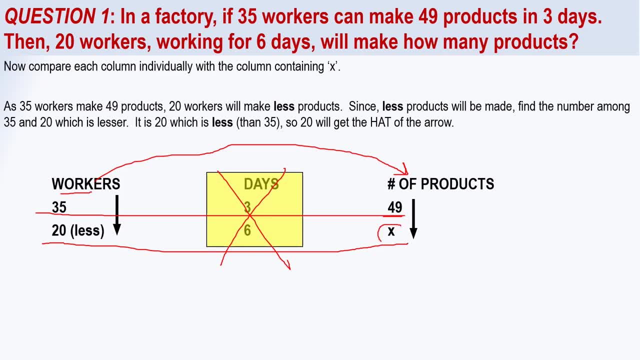 It is not important About 5. 처� también son 3. Up to 29. So suppose that 30 products produce how many products After 10.. And now that 30 will turn 2. Or the output will be less. 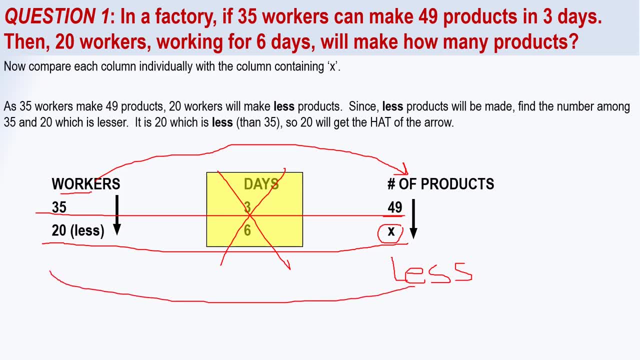 So it will be less. So the X is likely to be less. So we notice the word zero here because that is the likely value of X. So we take this less and we go back to this column and see 35 and 20.. 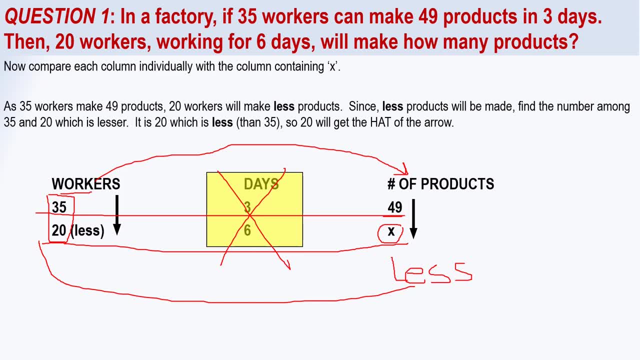 Which of these values is less. So we notice 20 is less, So we write less next to it And since it is less so, be given it a heir of the arrow. So this guide, 20 will get head of the arrow or head of the arrow, And we draw an error or an arrow, We draw pencil. 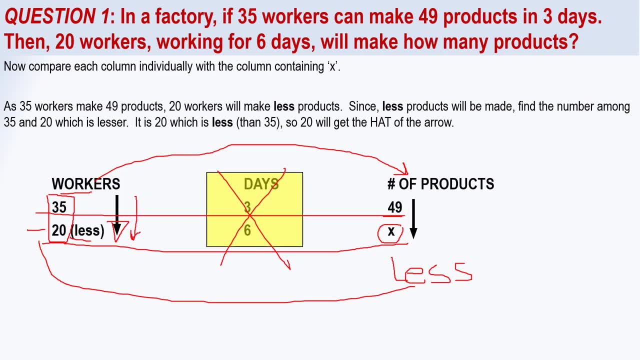 As to 60 words arrow. That gives 12 words. Each word is 20 words, So that used in 20 will receive 25 words, for which is pointing downwards. okay, so now we get to the next column. so we are now comparing the. 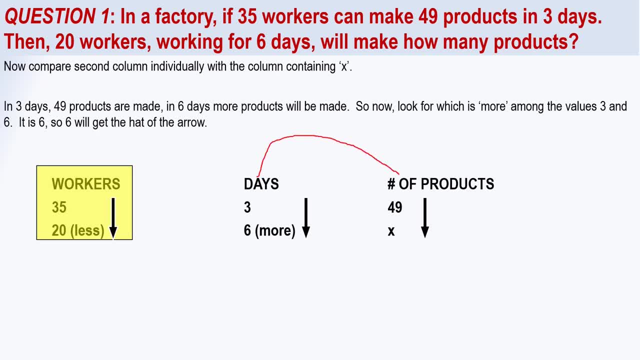 column which contains days and comparing it with the column which has number of products. so when we are doing it we should not worry about the workers column or any other column. so we just have shown it, kind of hidden. so we notice that in three days 49 products are produced, so in six days. 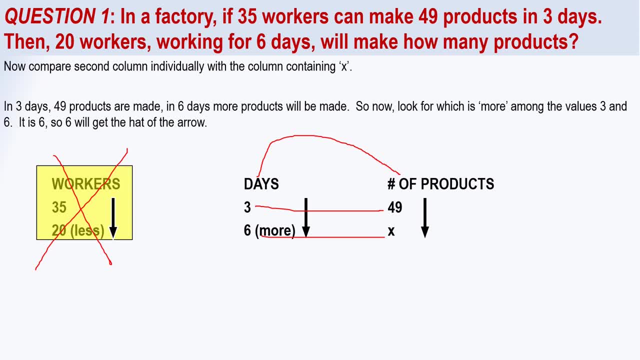 will there be more products produced or less products produced? obviously more products will be produced, so we think that the x will likely be more. so we take the notice a word more and we take this to the column here and we compare the values. the column in days has three and six. which of these? 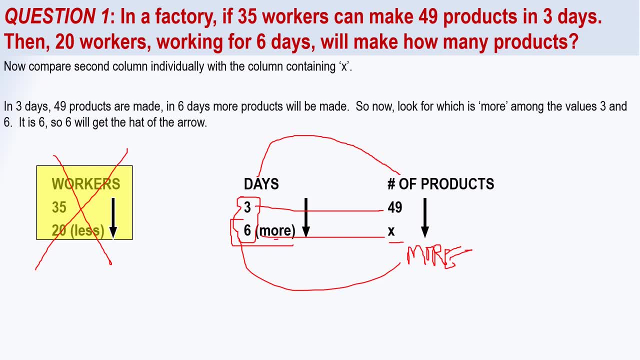 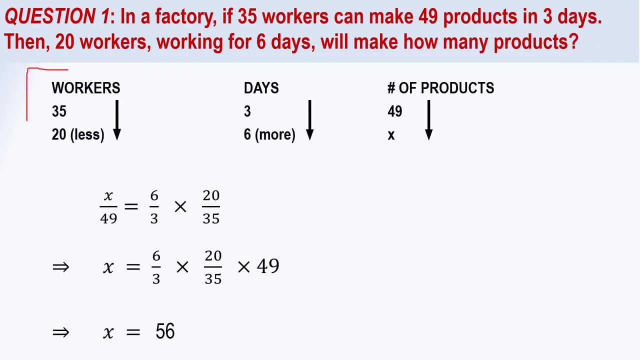 values three and six is more. obviously, six is more. so we write more here next to it and draw an arrow which has a hat or head pointing or kept in the position of six, that is, an arrow is drawn downwards. okay, so here we have our complete picture. that is, we have drawn the columns, we have filled them up with. 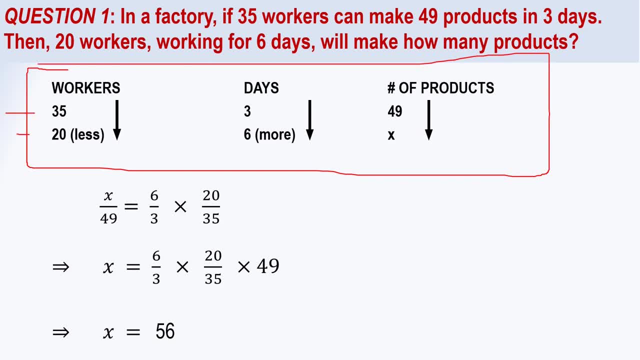 the values, that is, rows, and we have drawn our arrows for each of the column. the next step is that we have to create an equation in the equation. the first thing to note is that the unknown column, or the column which has x, is kept on one side of the equation, and all other columns are kept on the. 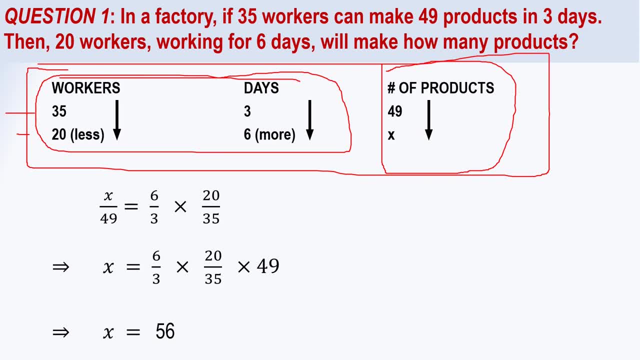 other side of the equal to sign or other side of the equation. the second point to note is this: the uh, the arrows, the head of the arrows, corresponds to a value that becomes the numerator and the values which correspond to the tail of the arrow become the denominator. so if you see here, let's say, 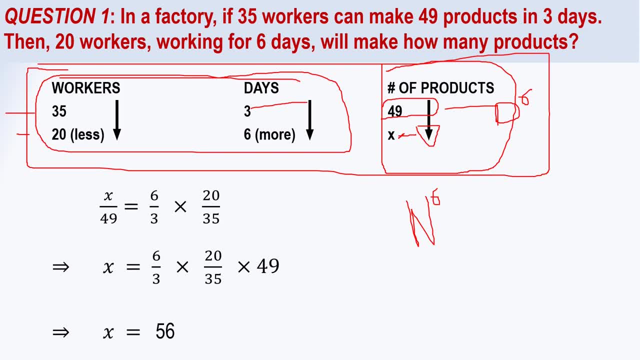 the days. column 3 has tail, so it will become the denominator. 6 has the head of the arrow, so it will become a numerator. then we write this equation as x divided by 49 is equal to 6 divided by 3, multi by 20 divided by 35. so here, if you see, the column which contains x is kept on one side. 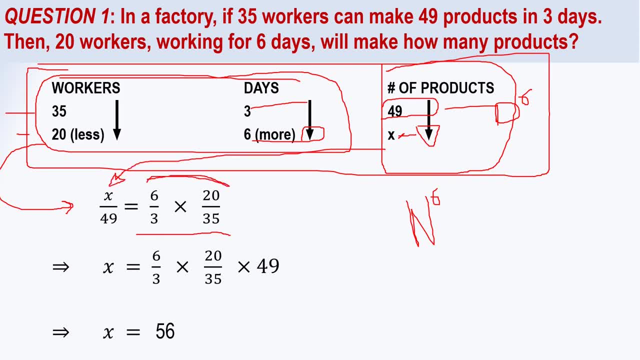 of the equal to sign. all other columns are on the other side of the equal to sign. x is having head of the arrow, so it becomes a numerator. 49 has the tail of the arrow, so it becomes a denominator. similarly, from the column of days we get 6 divided by 3, because 6 is the 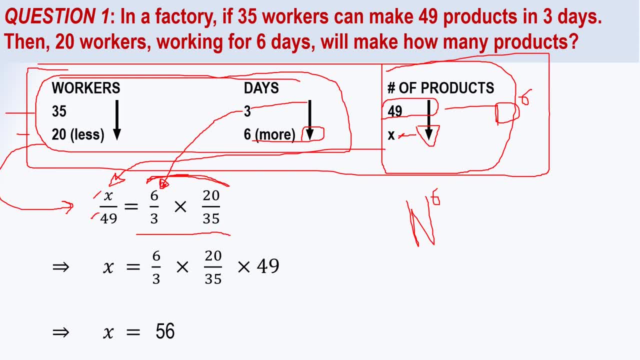 head of the arrow and therefore it becomes numerator. just like in the workers column, 20 becomes the numerator because it has head of the arrow. then we solve this equation and we get: x is equal to 6 by 3, multiplied by 20, by 35, multiplied by 49, which gives us x. 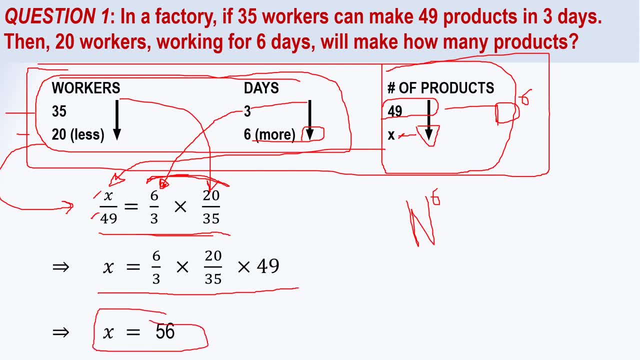 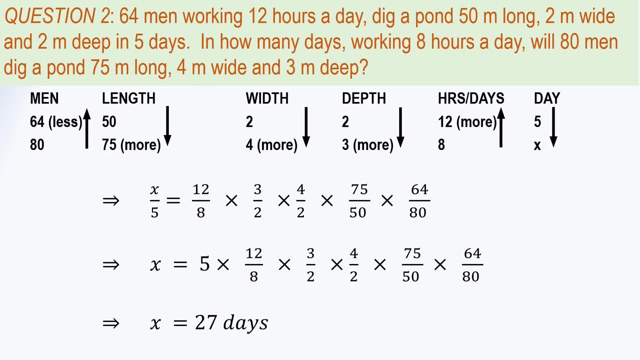 is equal to 56. that is, 56 will be the number of products as our answer. let's understand the arrow method using another example, which states: 64 men working 12 hours a day. take a pond 50 meter long, 2 meter wide and 2 meter deep in 5 days. in how many days? working 8? 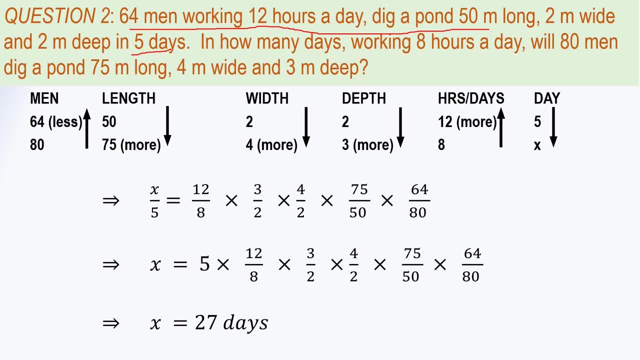 hours a day. a day will 80 men dig a pond which is 75 meter long to four meter wide and three meter deep. so we are given many things here, we are given men, we are given hours a day, we are given a pond which is of length, width and depth. so all those things that we are given will be converted into columns. 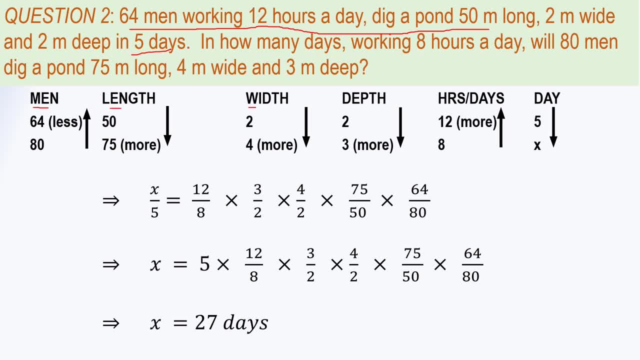 so we create columns for men: length, width, depth, hours per day and days, since we have to find in how many days. so we keep that to the rightmost column, because this is uh. this will contain an unknown. so once we have created these columns now, we shall have to fill up the columns rows into uh. 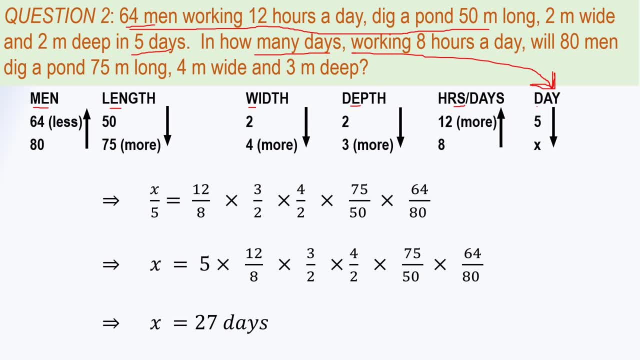 with some values. so we are given here 64 men working 12 hours a day. take a pound of 50 by 2 by 2.. so we put here 64 men length of 50, width of 2, depth of 2 and hours per day that they work. 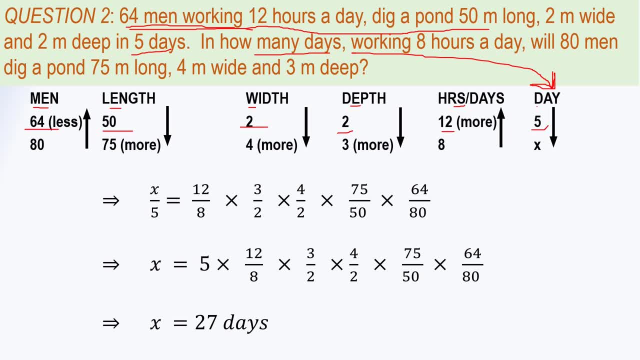 is 12 and they finish the job or create the pawn in five days, so that becomes our row number one. then we create another row which has men as 80, length as 75, width has four and depth has three and hours per day is eight, and it also contains an unknown, the 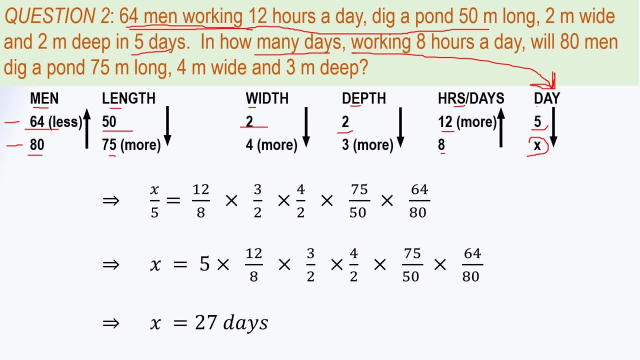 number of days that we have to find out. so, since it has unknown, we do not denote it by x and we create it in a column which is to the uh most, which is in the rightmost column here. now the next step is to start drawing the arrows. we start with the column which has unknown, which is x and the moment. 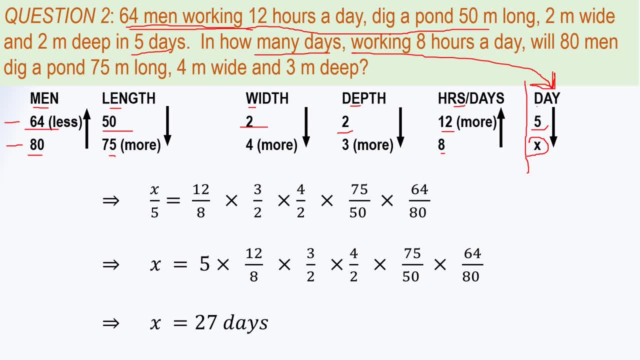 we see x. we draw an arrow which has its head or head at the x. so we draw an arrow which is downwards. okay, now the next step is to compare each column individually with the column which contains the unknown. so let's start with this column hours per day and compare it with the. 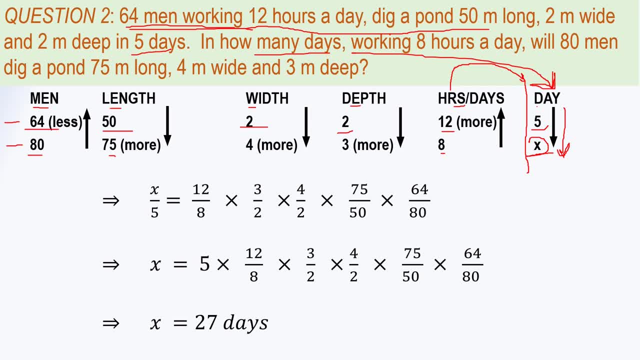 column which contains unknown, and while we do it we don't have to worry about any other column, so we can forget it or kind of hide it. so we see here now that 12 hours, if the work is done 12 hours a day, then the number of days taken is five. if the hours per day is eight, then obviously the same job. 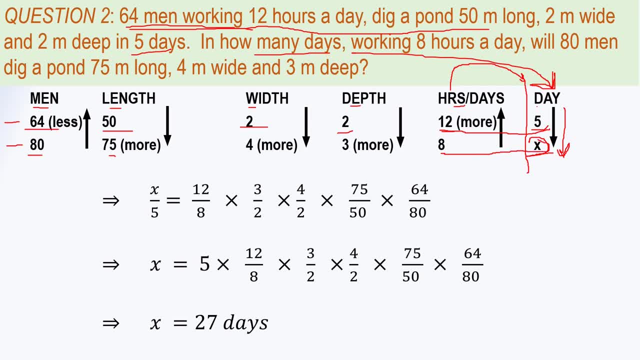 will be finished in more number of days. so we have to note the word more here and that is the likely value that x will take. x will take a more value now we take more to this column and see out of 12 and 8, which is more obviously, 12 is more. so we write more next to 12 and draw a arrow which has 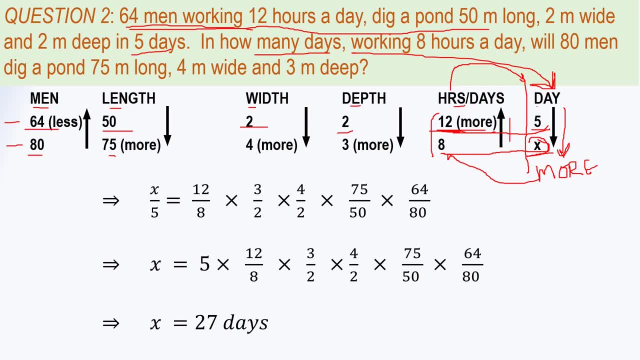 12, corresponding to the head of the arrow. so arrow is drawn upward so that the head or the head of the arrow is corresponding to 12 and the tail is at 8.. now the next step is to draw an arrow which is pointing downward so that head of the arrow is to the, or the head of the arrow is at. 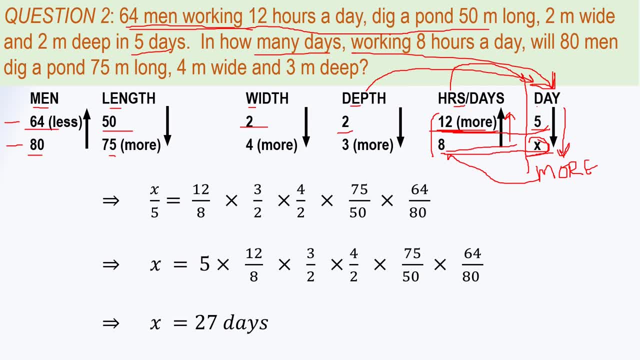 8.. now let's forget about this column of hours per day. let's go to another column and compare it with the column which contains unknown. so we go to the column of depth. we know a depth of 2 meter is done in five days. then depth of 3 meter will be 10, obviously in more days. so we note the word more. 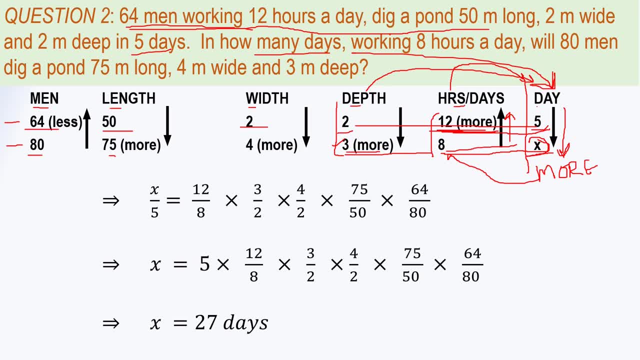 bring it here to the column which is column of depth. we see the values 2 and 3. which of these two is more? three is more, so we write more next to it and we draw an arrow which is pointing downward so that head of the arrow is kept at 4.. similarly, we compare width column with the unknown column. 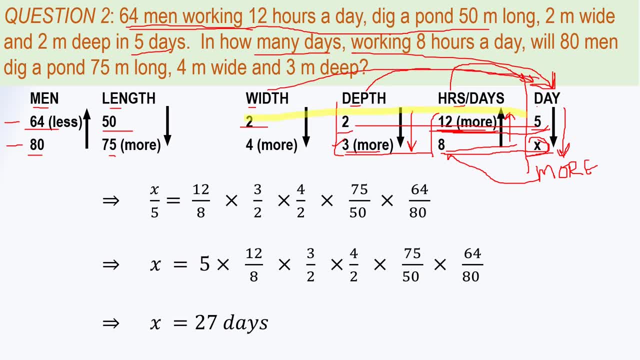 and we see that the width of 2 is built in 5 days, so width of 4 will be built, obviously more days. so we write more here, uh to the uh, more here to here to in this column: uh, because 2 and 4, if we 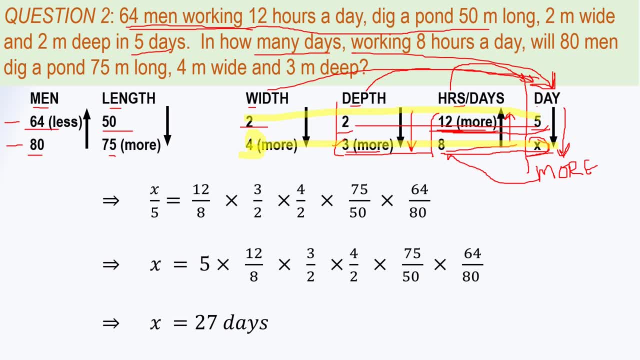 compare: 4 is obviously more. so we draw an arrow downwards so that the head of the arrow is kept at 75. so we draw an arrow downwards so that the head of the arrow is kept at 75.. similarly, we compare length and days. uh, we know that 50 length is done in five days. 75 will obviously be done in more days. 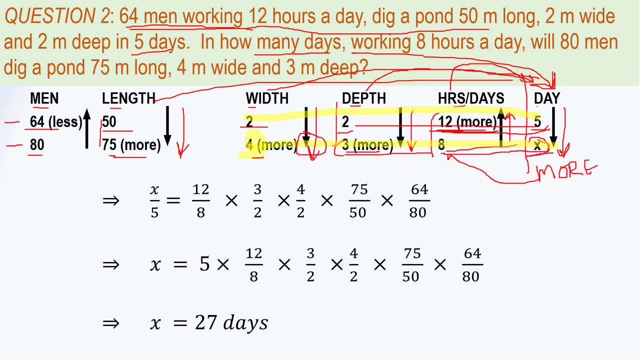 so 75 is more out of 50 and 75. so we draw an arrow downwards so that head, or the head of the arrow, is at 75.. similarly we go to the final column of men. 64 men can do the job in five days, so 80 men will. 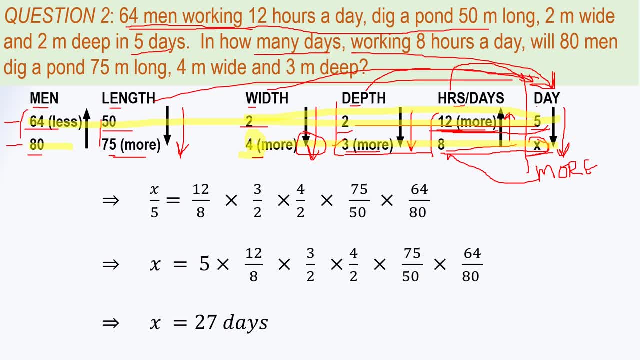 obviously do the job in less number of days, so we take the word less and then compare it. in this, 64 is less than 80, so we will draw an arrow which has its head at 64.. so now we have drawn all the arrows, we have completed our columns and their rows, so next step is to write the equation as we. 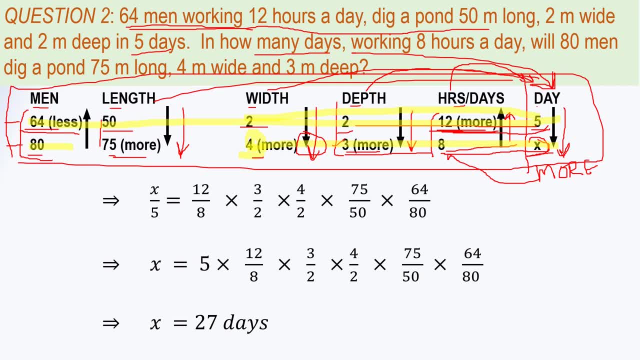 know, all the values which have head of the arrow become the numerator and all the tail values become the denominator. and the second thing is that the unknown column is on one side and all other columns go on to the other side. so we get an equation where x by 5 is equal to 12 by 8. 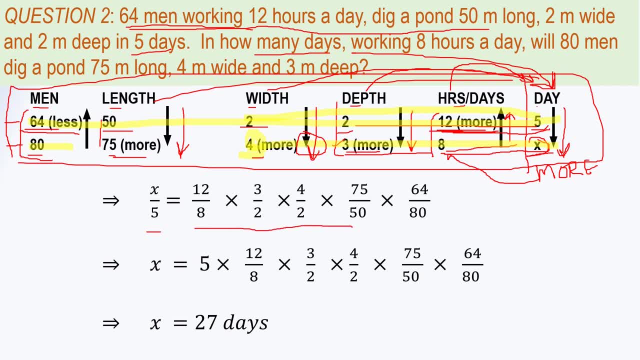 multiplied by 3 by 2, multiplied by 4 by 2, multiplied by 75 by 50, multiplied by 64 by 80, when we solve it, we get: x is equal to 25 days, and that is our answer. if one man or two women or 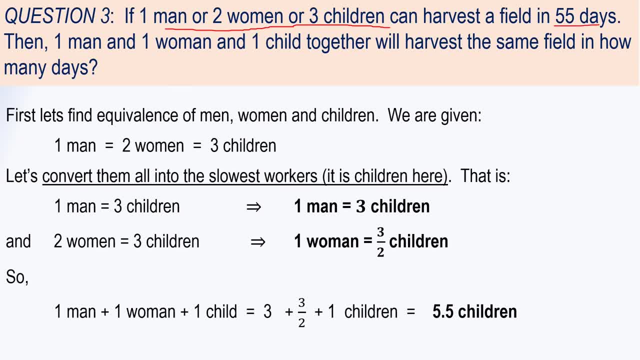 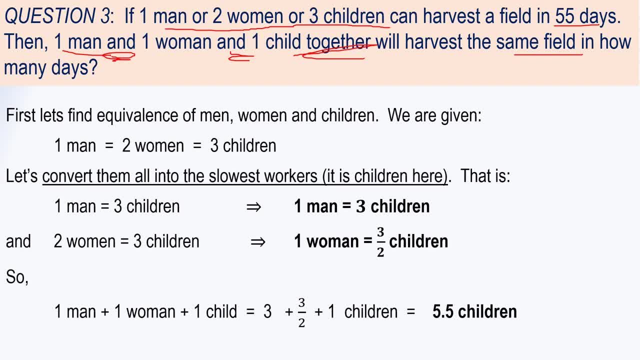 children, and men and children like that. so here we are, given either one man or two women or two children, so we can say that one man is equal to two, women is equal to three children. now let's convert them into children. why we are converting it to children is that it appears to us very 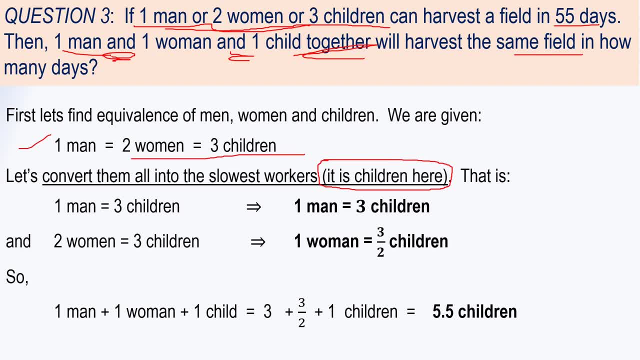 clearly by reading the question that children are the slowest. so it's always good to- it's good for the sake of ease in the calculations that we convert them all into the slowest worker. so we convert men into children and we get: one man is equal to three children and two women is equal to. 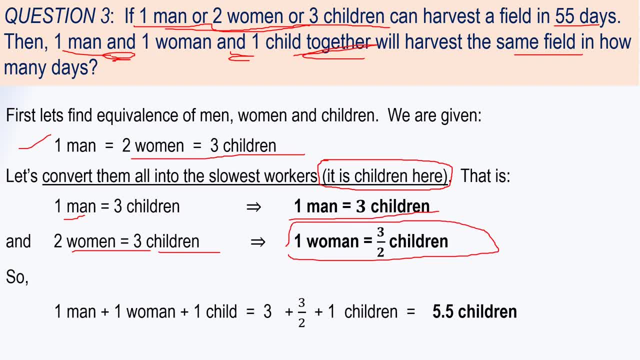 three children, which implies one woman. woman is equal to one and a half children. so now, if you see, in the question we are asked how many days will it be taken by one man plus one woman plus one child? so we keep it and here so we get: one man plus one woman plus one child is equal to: 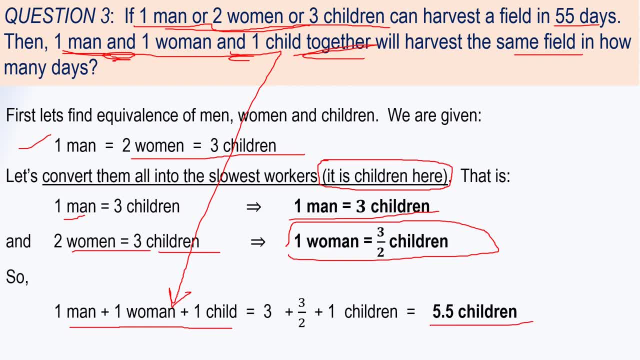 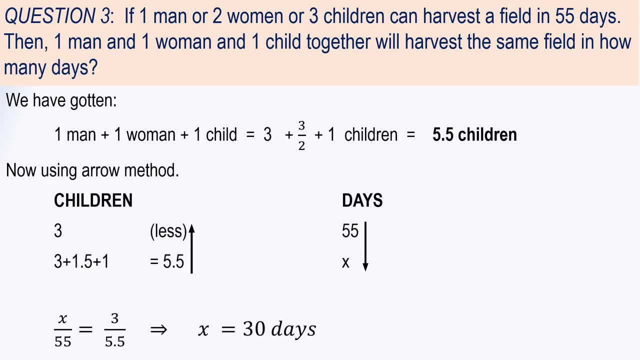 we convert them into the terms of children and we get 5.5 children. okay, our next step is that. our next step is that we convert them into children and we get 5.5 children. after having gotten the equivalence is to draw the columns and draw the arrows. so now we have. 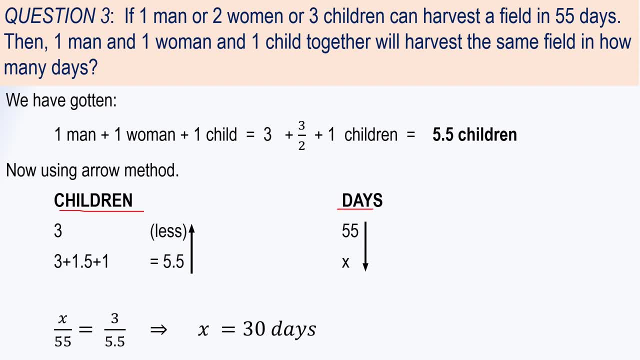 converted everything into children and days, so we have only these two columns. so we are given that three children can complete the job in 55 days, because that's how we are given one man or two women or three children, and the other is that what we have to find out is that 5.5 children 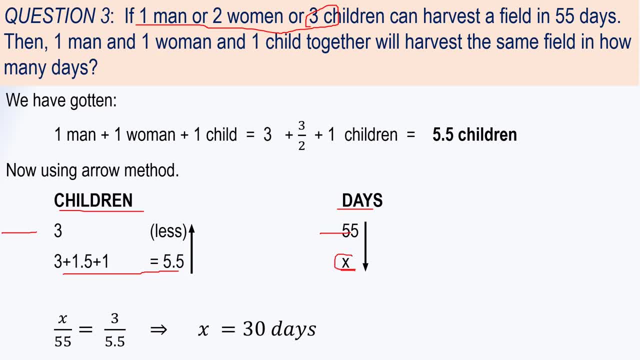 will do the job in how many days. so our unknown is number of days. therefore we have kept it in right: most column here. other column that we have is of children. so three children do the job in 55 days. so 5.5 children will do it in the less, less days. so now this less days, we take the word less. 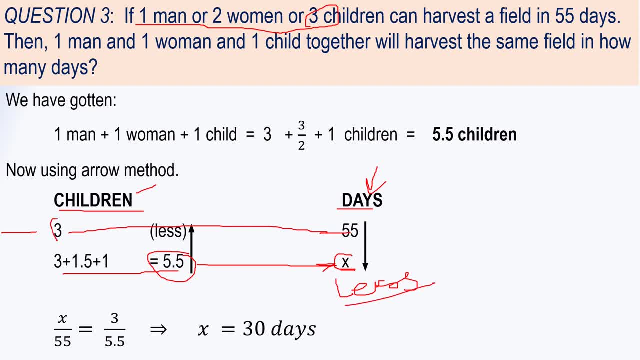 and take. compare the values 3 and 5.5, whichever is less here. in this case it is 3 which is less, so we draw an arrow upward so that 3 gets the head of the arrow and then we solve it. x goes the numerator, 3 goes in the numerator. 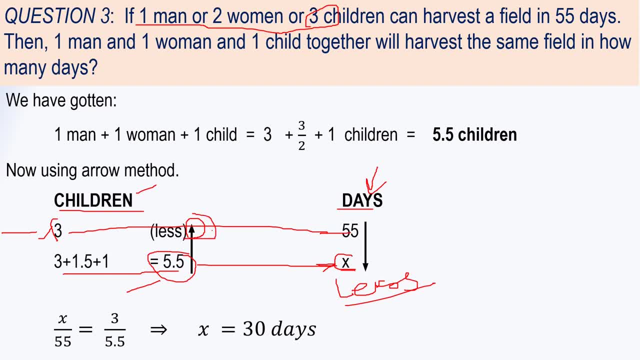 because 3 has head of the arrow. other values go in the denominator and we solve it. x by 55 is equal to 3 by 5, by 5.5, which gives us x is equal to 30 days. and that's our answer. let's do another. 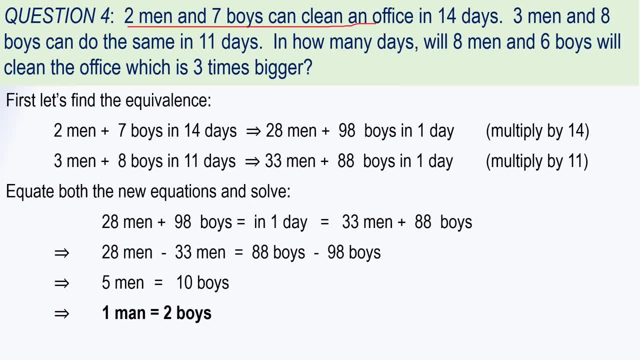 question. question number four, which is, two men and seven boys can clean an office in 14 days, then, and also three men and eight boys can do the same work, that is, cleaning the same office in 11 days. now the question is: in how many days will eight men and six boys will clean the office? 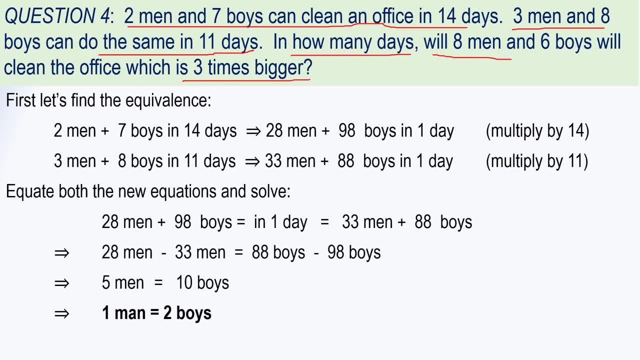 which is three times bigger. so let's, as we did in the previous question, let's first find the equivalence. so we are given that two men along with seven boys can clean the office in 14 days. so if we multiply this by 14, so we get 28 men plus 98 boys can do the work in one day. we are also 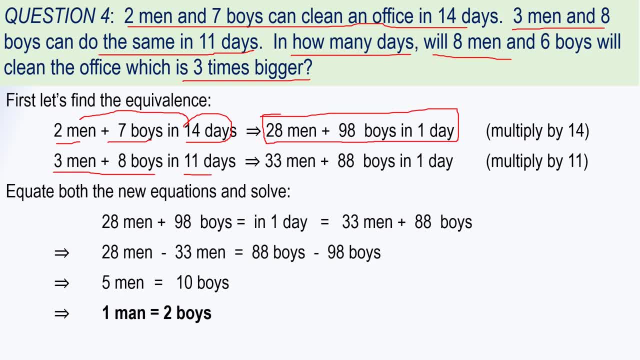 given, the same office can be cleaned by three men and eight boys in 11 days. now we multiply them by 11 and therefore we get that 33 men and 88 boys can clean the office in one day. so here, by multiplying, we have gotten everything here in the terms of one day. okay, now we equate these. 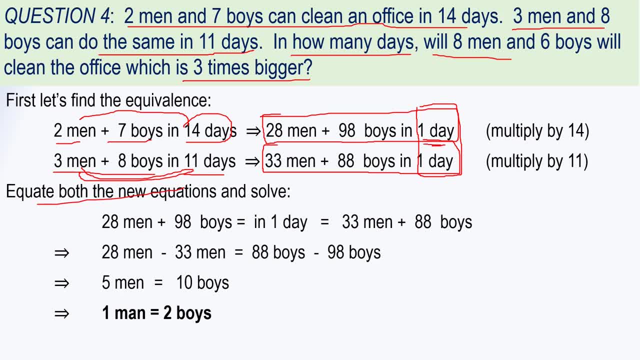 equations, because this is one day. the job is done in one day by 28 men and 98 boys. same job is done by 33 men and 88 boys. so if we equate them so we get: 28 men plus 98 is equal to 33 men plus 88 boys. 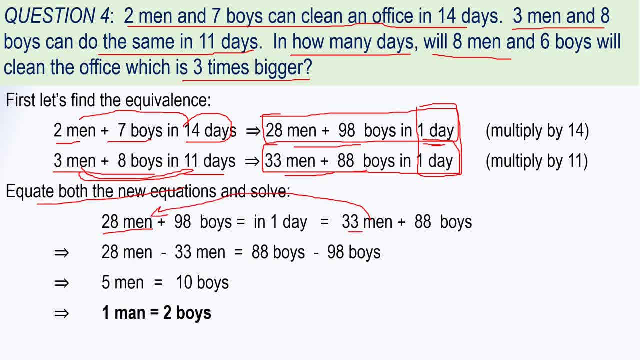 and now we take men to the other side and boys to the other side, so we get 28 men minus 33 men, which is equal to 88 boys minus 98 boys, which implies one man is equal to two boys. okay, so now we have already established that one man is. 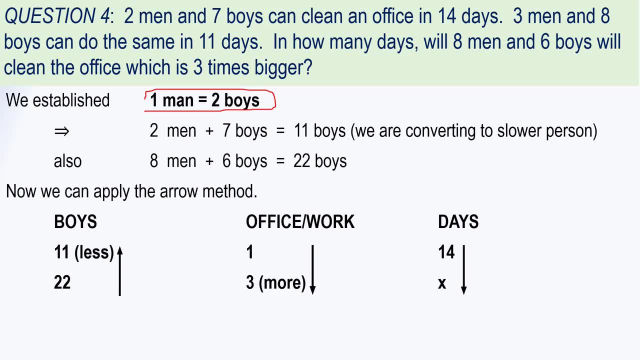 equal to two boys. so we know that which we are given already, that two men and seven boys can do the work in 14 days. so two men plus seven boys is equal to how many boys, which will be equal to 11 boys. so if we were to solve this question by creating our 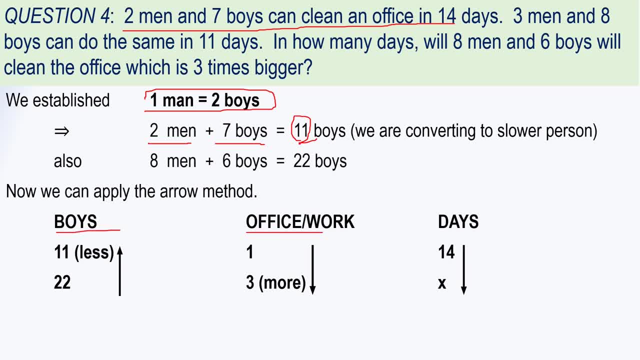 columns. so we will create the columns of boys, we create the column which of the work, and then we create the column of days. we are given that the 11 boys, 11 boys is coming from here, 11 boys do the one office cleaning up in 14 days, and then we are asked that 22 boys because 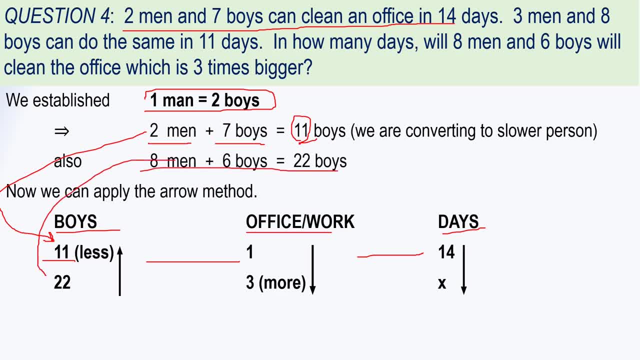 we have converted 8 men plus 6 boys into 22, so 22 boys will do the three times the work or the office which is three times bigger. they work in how many days. we denote it by x. so this is how we have drawn our columns. and again, since x is here, x gets the. 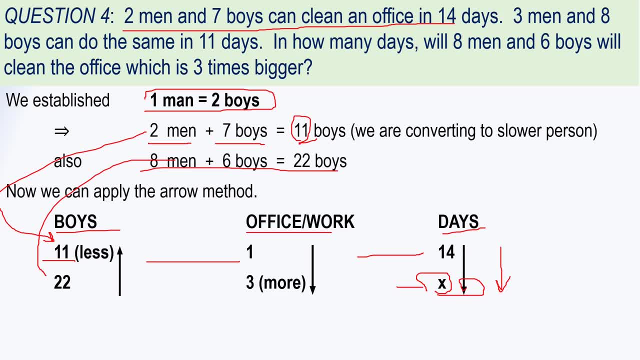 head of the arrow. so we draw an arrow which is downwards. then we look at the office work, compare each column individually with the column containing unknown. so we know one work is done in 14 days, so three work will be done in more days. so we take the word more and we take it to the columns value. 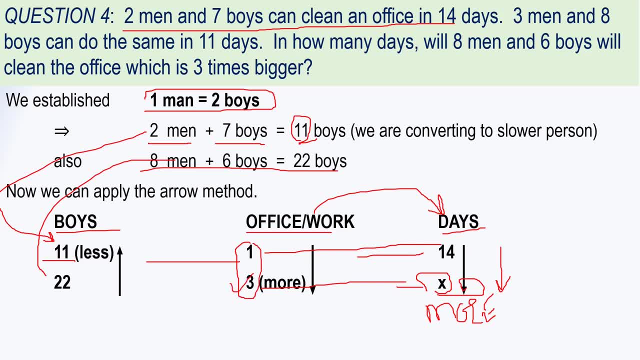 one and three. which of these one and three is more? obviously, three is more than one, so three gets the head of the arrow and we draw an arrow downwards. similarly, comparing it with the boys column and forgetting about this column for the moment, we see 11 boys do the 11 boys do the work in 14 days. 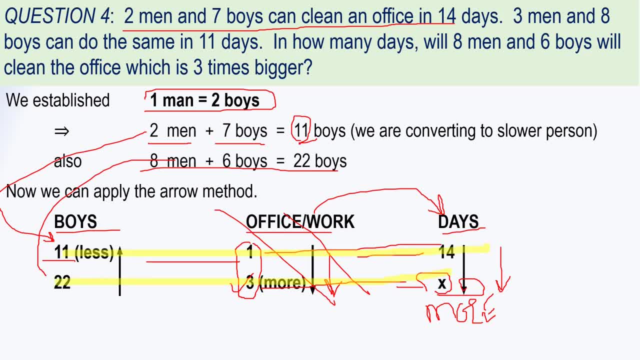 and then 22 boys will do the work in obviously less days. so we take the less word and out of 11 and 22, which is less, 11 is less, so 11 will get head of the arrow. so we draw an arrow upward like this: